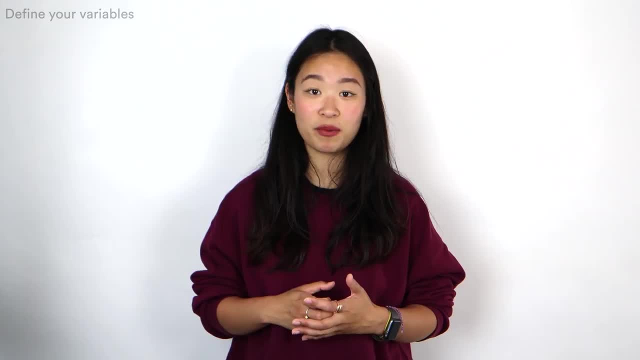 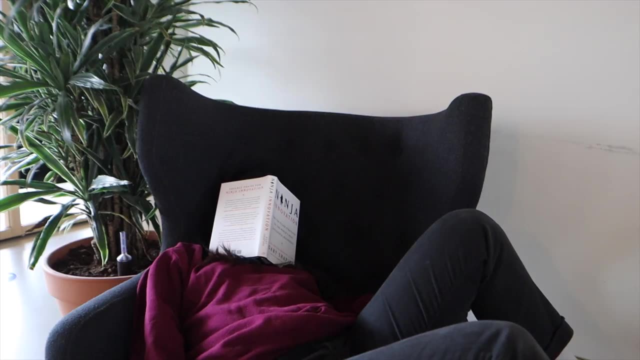 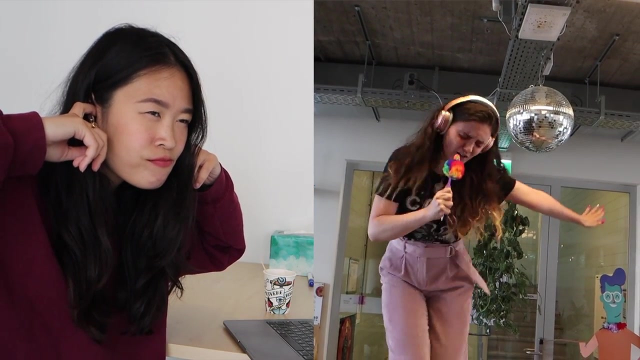 You'll also need to control other variables that could affect your dependent variable outcomes. In our example, you might control the amount of sugar in the drinks, the time of day you test participants and the test environment, because these can all affect memory test performance. 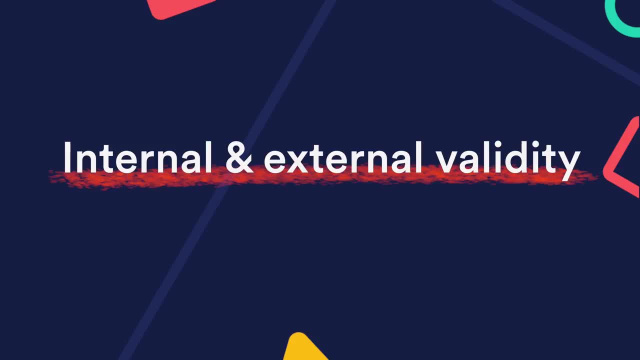 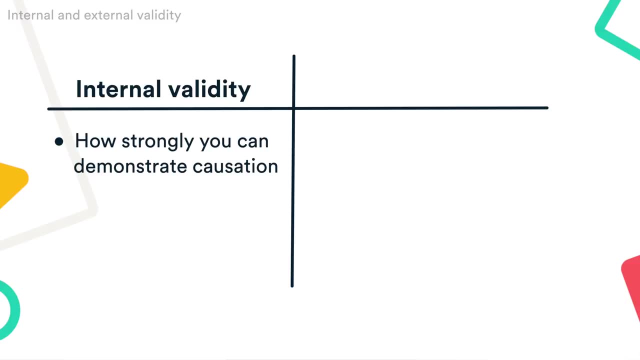 As you design your experiment, you'll need to strike a balance between internal and external validity. Internal validity is about how strongly you can demonstrate causation. You'll need to make sure that nothing other than your manipulation can explain your outcomes. External validity is about how confidently you can generalize your findings to broader populations or real-life settings. 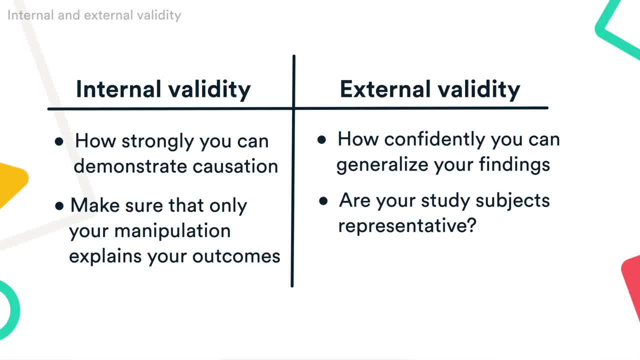 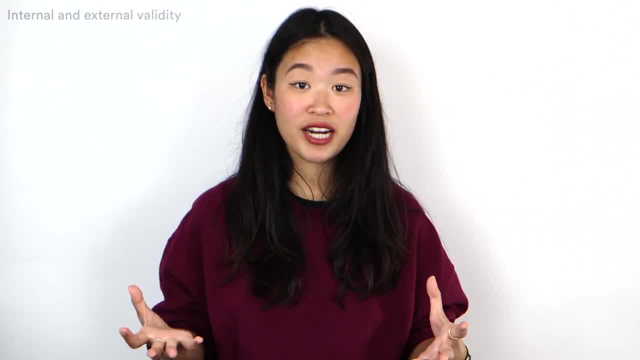 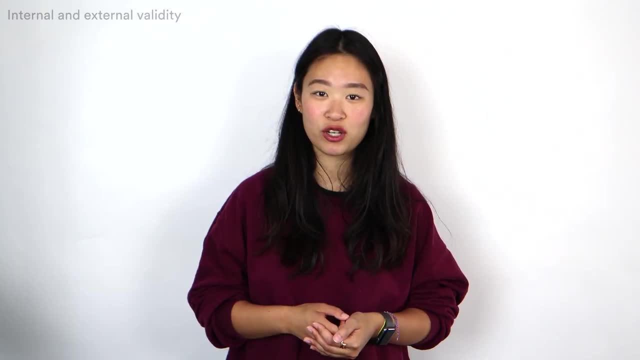 Are your study subjects representative of the population you're interested in? Is your study environment similar to the context you apply your findings to? There's a trade-off between internal and external validity. Experiments have higher internal validity than other types of research, but they often have lower external validity. 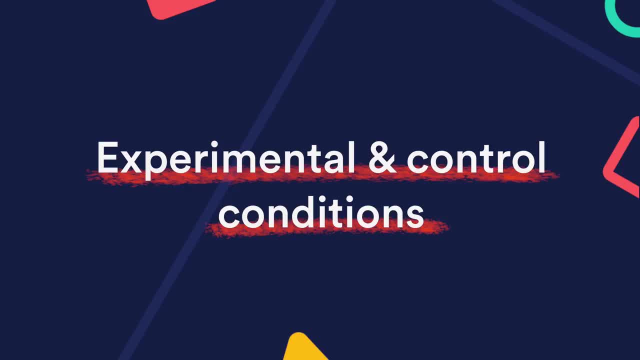 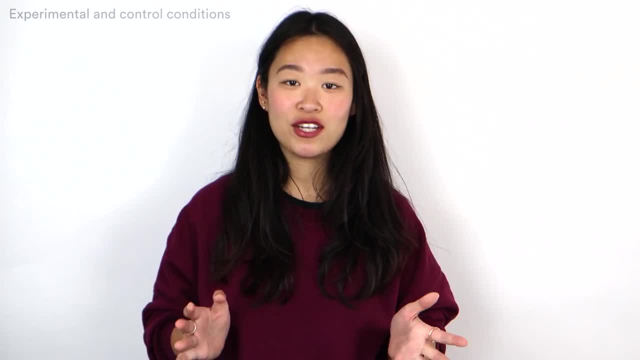 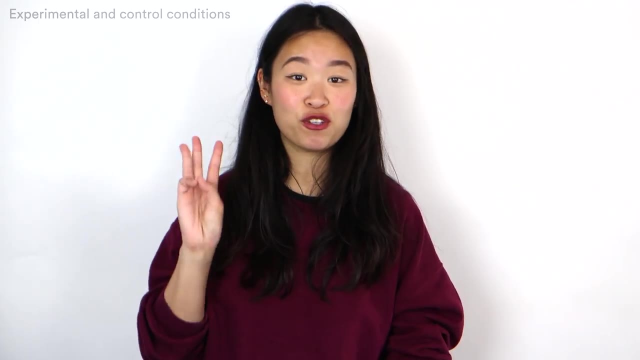 To manipulate your independent variable, you'll create two or more conditions. These are sometimes also called treatments or levels of the independent variable. You need to decide how many conditions to use and how widely they will vary. For example, in your caffeine experiment, you could use three conditions. 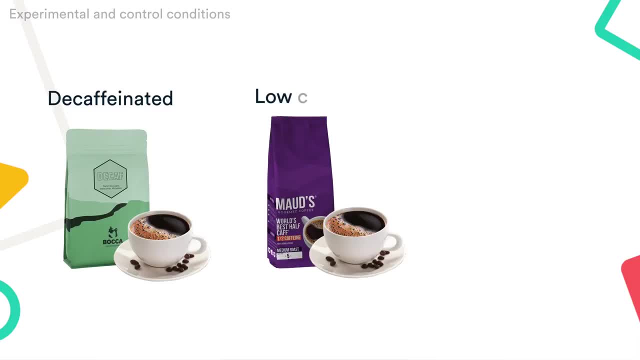 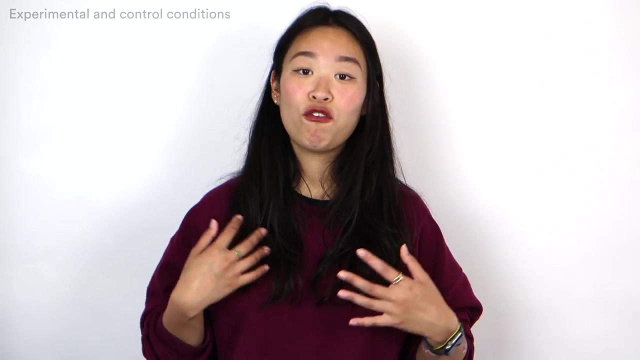 Participants will receive drinks with either no caffeine, low caffeine or high caffeine. For internal validity, you need at least one control condition to compare with your experimental conditions. In our example, the control condition is no caffeine. For external validity, you'll need to consider how well your conditions reflect real-life settings. 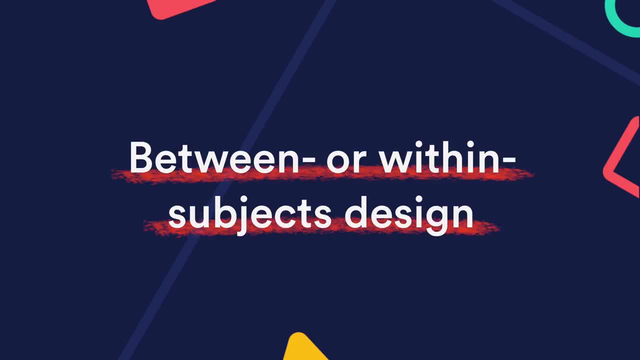 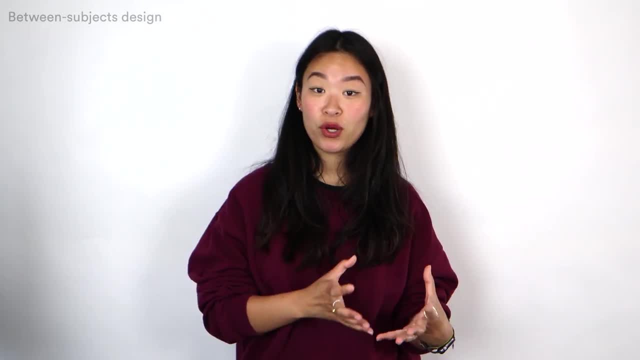 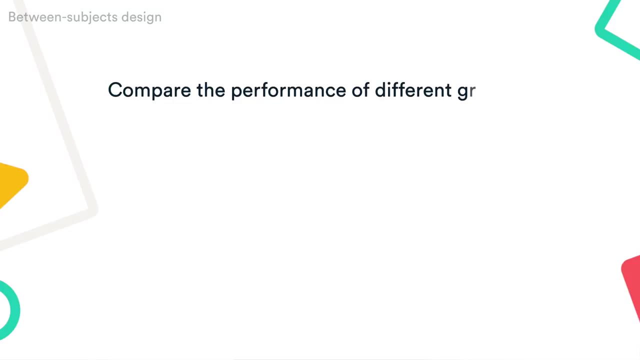 In your experiment you'll compare different conditions with each other, But first you need to decide whether you'll compare these between or within groups A, between groups or between subjects. design means that each subject will only experience one condition. In our example, that means you have three groups. 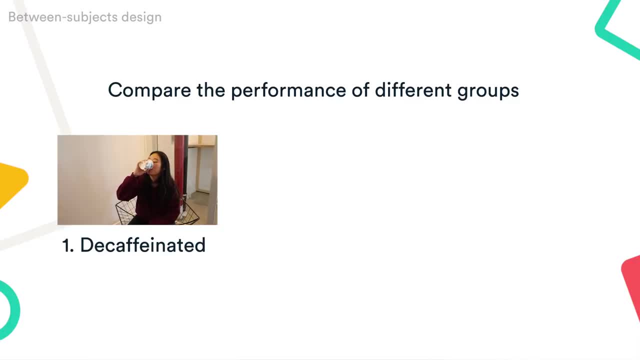 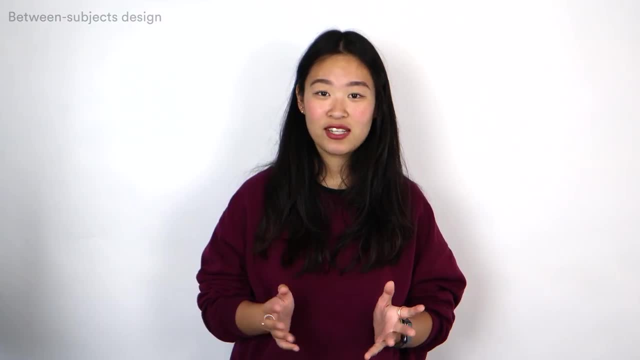 Group 1 receives a decavenated drink, Group 2 receives a low caffeine drink and Group 3 receives a high caffeine drink. Participants are placed into one of the three groups at random and you compare the short-term memory performance of these different groups.